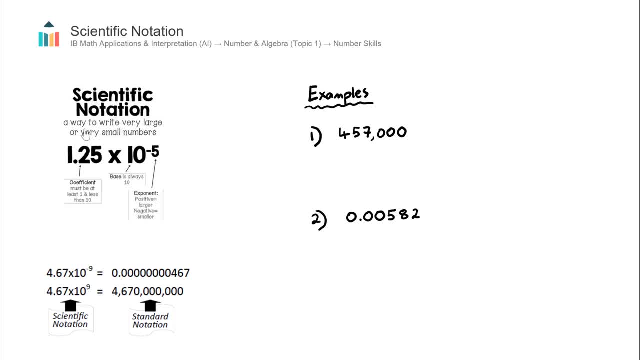 notation. Now just to recap. scientific notation is a way to write out very large or very small numbers. rather than have to write out all of the digits, like we can see here in the bottom right, we can write them in a more concise, compressed form, like you can see here on the left hand side. 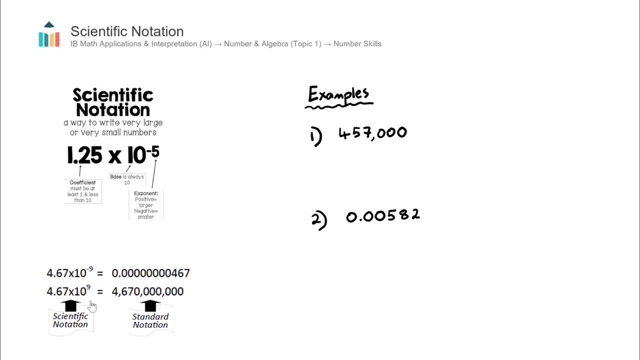 So very, very useful. If you're writing out, say, the distance from the earth to the sun, that's a very, very long number. or maybe the diameter of a cell in the body. it's a very, very small number. It's easier to actually write it out in scientific notation. 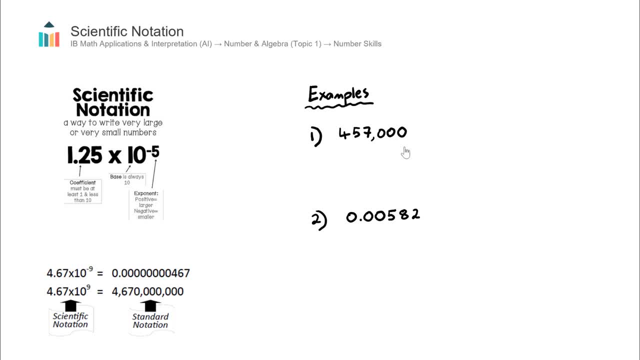 Okay, let's work through these two examples here. the first is a large number and the second is a small number. So this first number here- 457,000, is currently in standard form and I'm going to convert that into scientific notation. 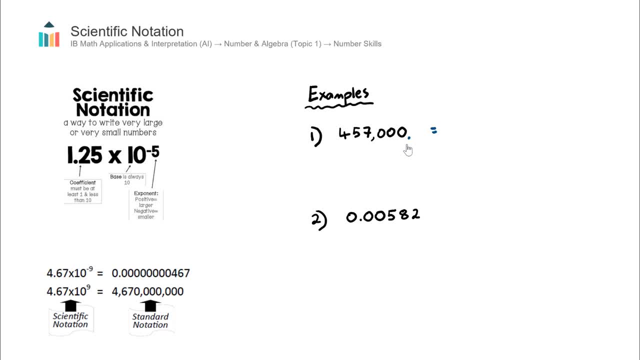 Now, currently, the decimal point is at the right here. whenever it's a whole number, the decimal point is on the right hand side. Now the trick- well, not so much the trick, but the way to go about converting numbers into scientific notation- is to think through: how many times does the decimal 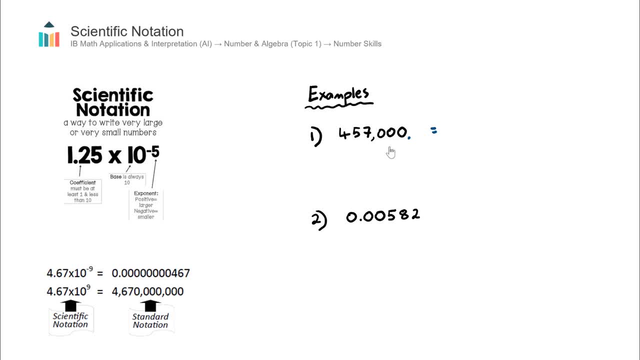 point need to move such that this number here becomes a number between 1 and 10.. So for example, 4.57 as opposed to 457,000.. Well, the decimal point needs to move once, twice, three, four, five times. So just remember that number five times. 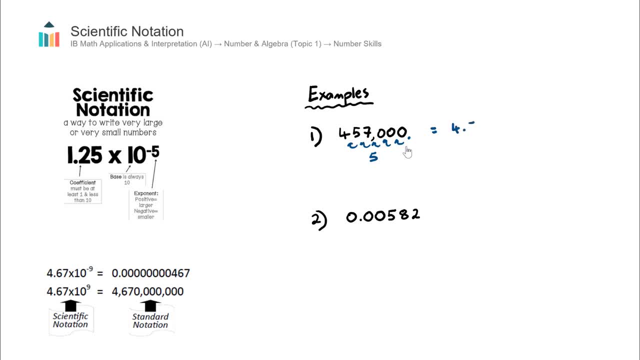 So this number here will become 4.57,. I have converted this number into a number between 1 and 10, and the form of scientific notation is always times 10 to the power of, and the power is whatever number I have here, the number of decimal place movements. 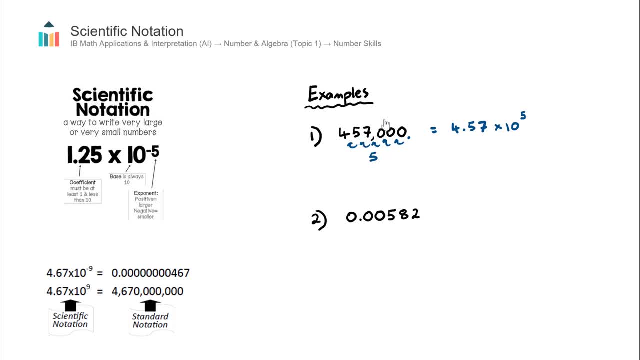 So the power of five. Now, because this is a large number, the power or the exponent will be positive. If it's a small number, like the second example here, which we'll get to in a second, the power will actually be a negative number, Just like you can see here in the bottom left. 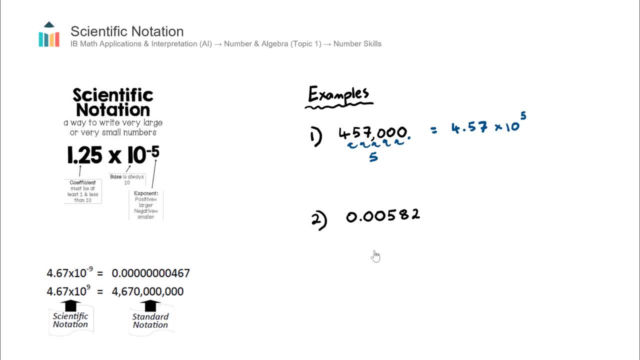 this is a very small number. the power is negative. Okay, let's try the second example. Again, let's think through. how many times does the decimal point need to move in order for this to become a number between 1 and 10.. 5.85..